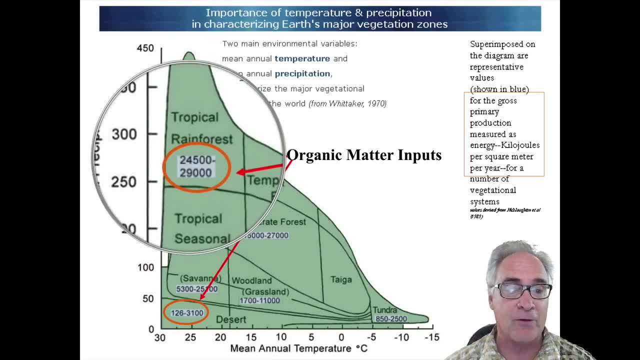 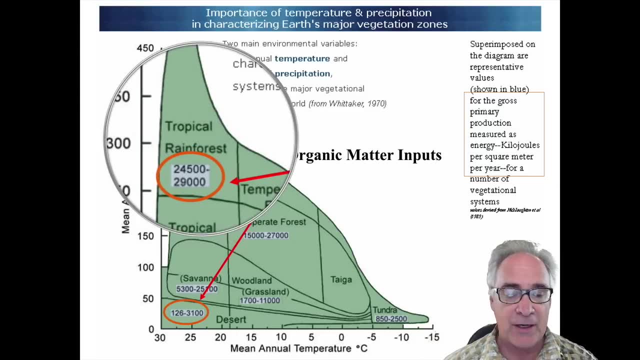 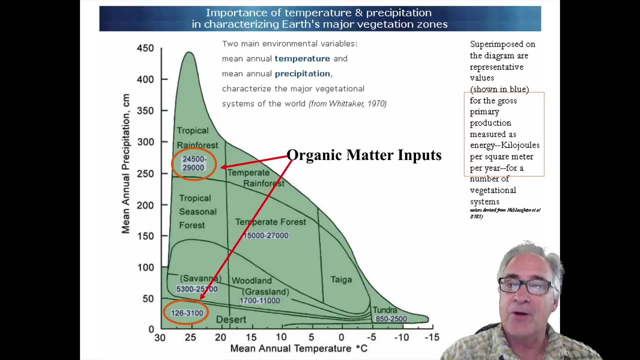 graph. And let me see here. Let me go ahead and put it right. If you look right here, tropical rainforests have the highest amount of energy per acre than anything else, where the lowest is the desert. And why is that? Well, it's the combination of high temperature and also high 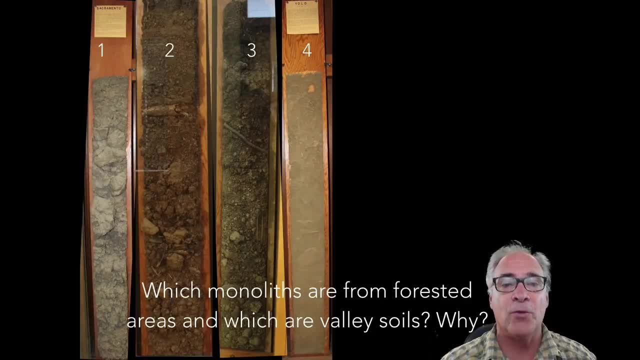 precipitation. We have four soil types. They're here from California and in particular kind of around the Central Valley area, And could you tell me which ones are from forested areas, areas that have organic matter and also have a lot more rain than, let's say, the Valley. So take a second and tell me which two. 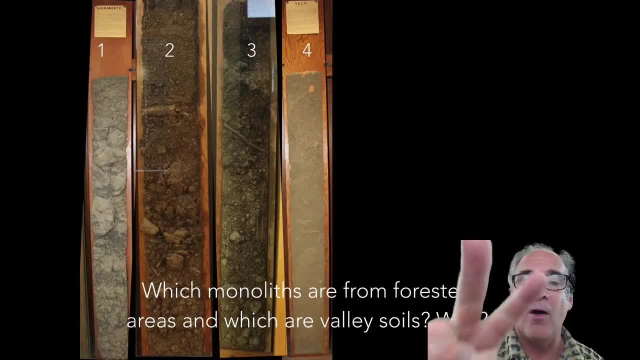 of them are from the Valley and which two of them are from the forested area. So let's take a look. So the forested area. if you said 2 and 3, you'd be right, And if you take a look at 2 and 3, you'll notice first. 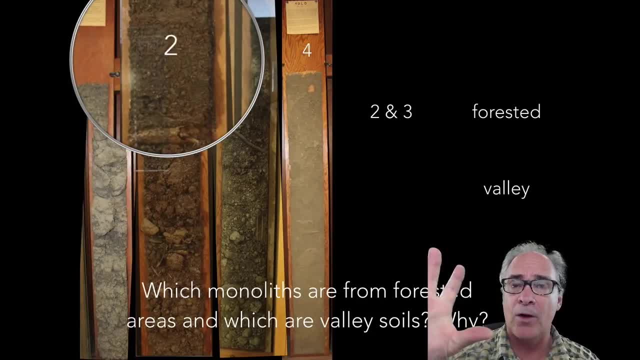 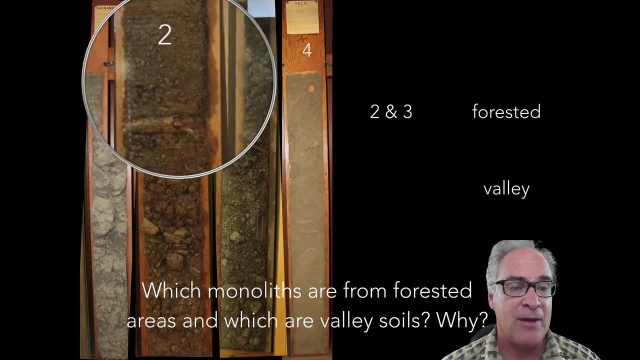 of all the darker color, which means there's more decay and more of the organic matter making it's way in, especially a lot of the tannins, if they're around things like oak trees and, and if you take a look here, here's an acorn. that's. 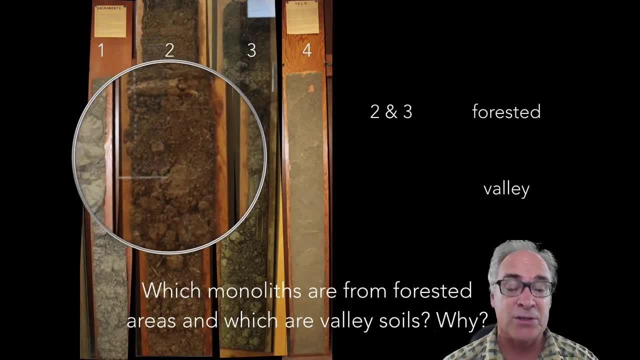 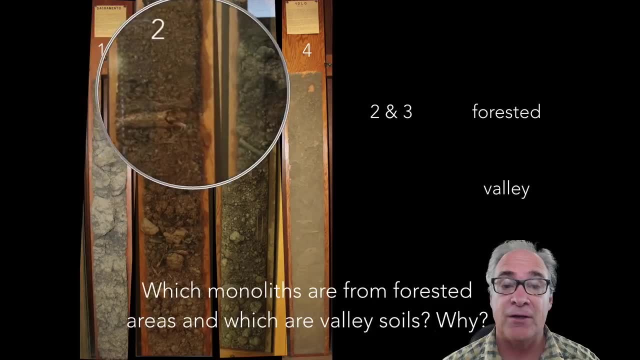 stuck right there about six inches in, and you see roots and remnants of roots even far down into the b horizon. so that's definitely a four from a forested area, and then one right here. if you take a look at number three, you'll notice that little kind of band of kind of lightly colored. 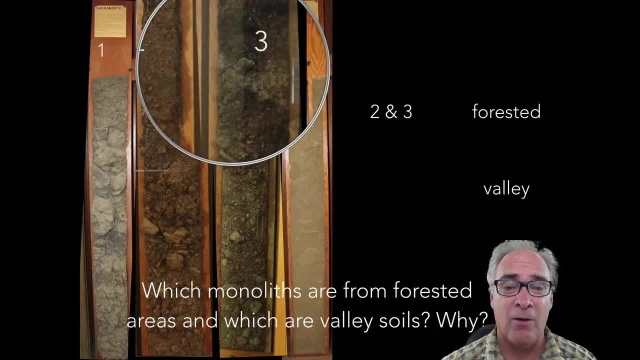 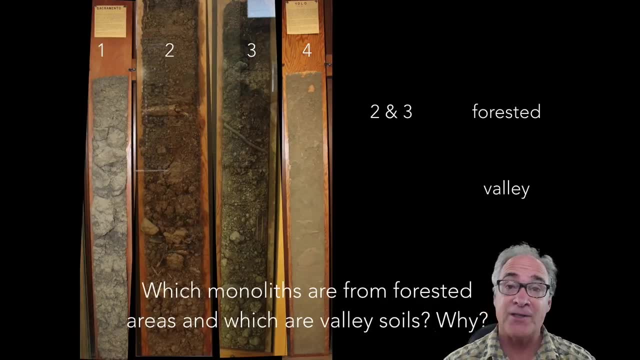 soil, that's some clay, so that's an e layer or e horizon, and you have twigs and you have some more roots in there. so yeah, two and three are from forested areas that get a little bit more water, actually a lot more water, and of course, because of that, they have many more trees, which has more. 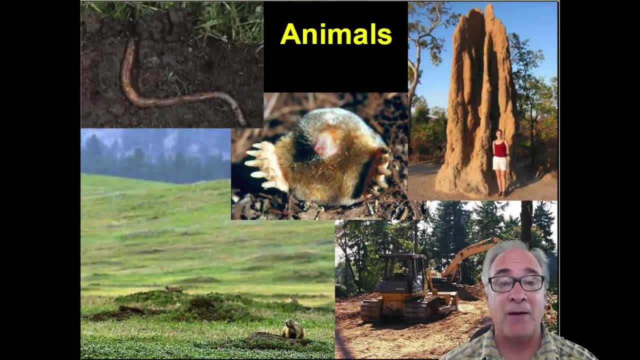 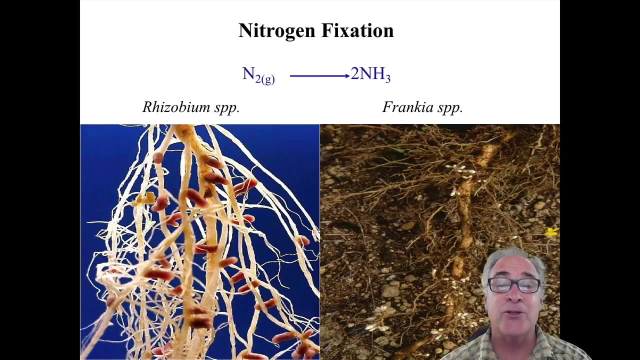 organic matter now. animals have a tremendous impact because they keep mixing and moving soils and and adding things such as manure and other kind of nutrients within the soil. if we first of all take a little bit of animals and microbes, you'll notice that nitrogen fixation happens in. 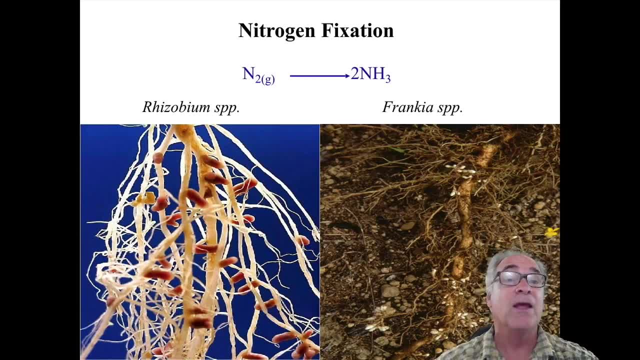 landfills and in the soil. so that's a little bit of that. and then you have a little bit of nitrogen fixation happens in landfills and in the soil. so that's a little bit of nitrogen. fixation happens in legumes and while it's in the soil it will release some of those uh nitrogen compounds. 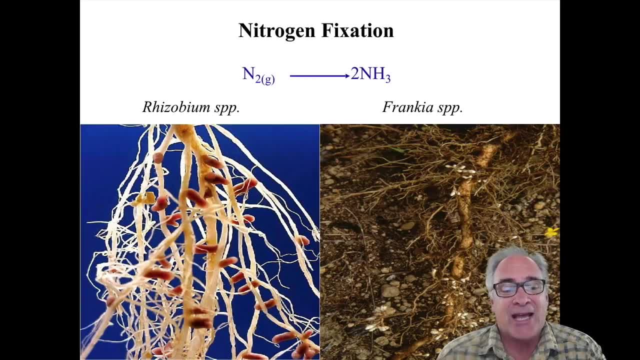 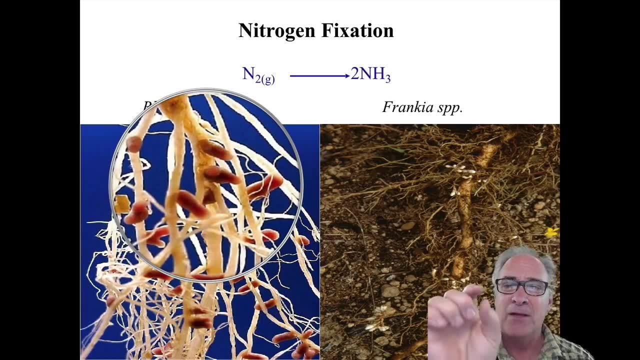 and nitrates and the ammonias and of course the nitrogen gases is kept in these little nodules. uh, these little nodules that are right there, those little things are nodules. they have bacteria in them that actually help manage the nitrogen cycle, and then even trees and cars, of course, getting 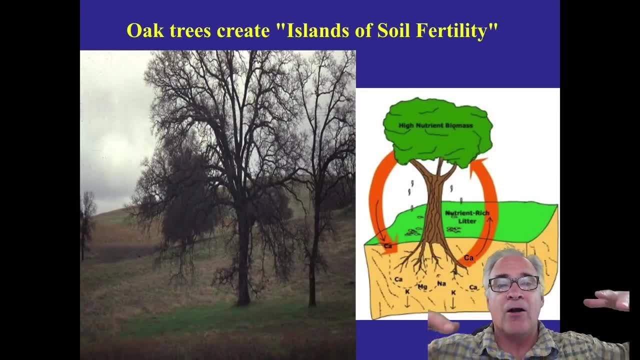 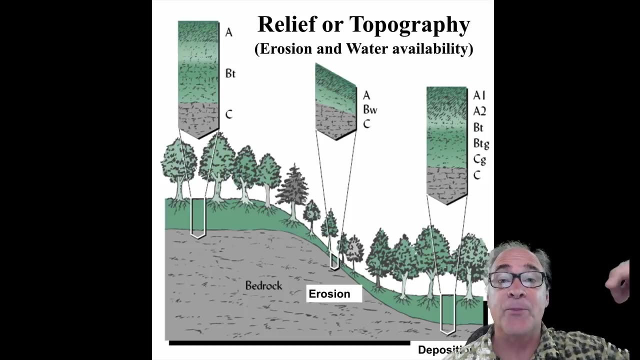 into the action, oak trees in particular. they are a terrific, terrific generator of all kinds of organic matter. i have a huge 300 oak tree just on the side of my house. it's constantly dropping stuff. now we get to all the r factor or topography, the way that the ground 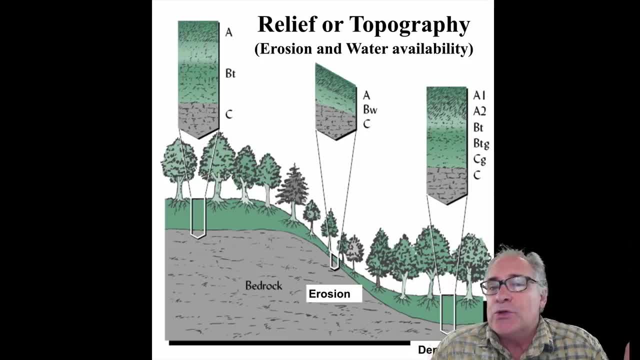 is shaped. so when we look at topography, it has a huge impact on the profile. for instance, up in the sierra is the highest part of our cross section through california. you'll have all three of the topography. you'll have a fairly thick b layer and, of course, the c layer, and that's fairly stable. so 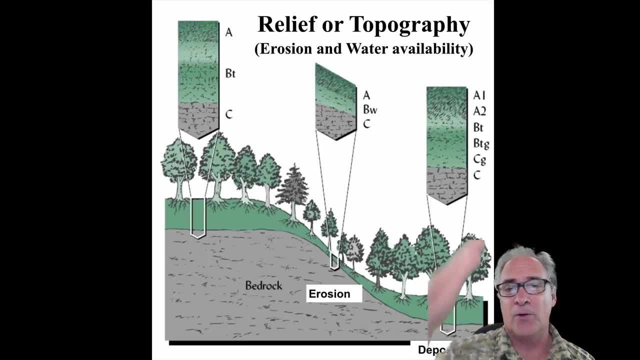 those are the oldest soils you're going to find here in california. if you cross section from east to west in the slope or the foothills you're going to notice a, b and c layers, but the b's and the a's are kind of thin because of uh erosion it's. it is always kind of in the pathway some kind of erosion. 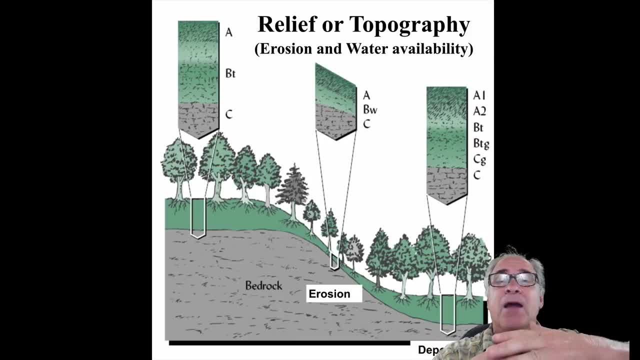 whether it be water, whether it be wind, and then the valley floor, you have uh also very, uh much thicker, thicker soils. in particular, the topsoil tends to be a little deeper, the the b or subsoil tends to be uh deeper as well, because um and and different kinds of soils too, primarily, 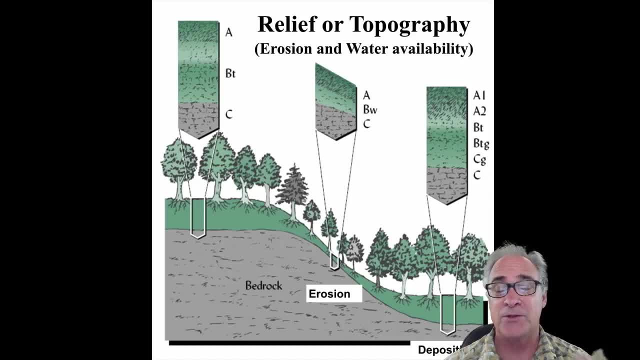 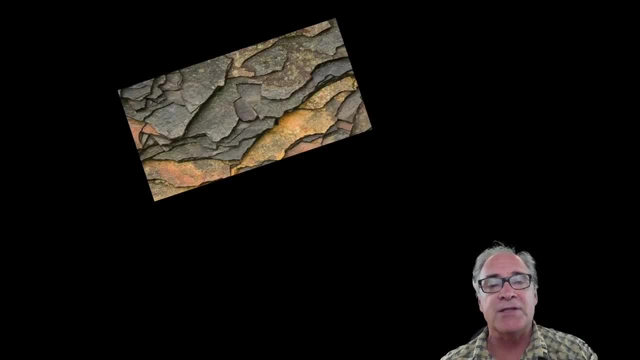 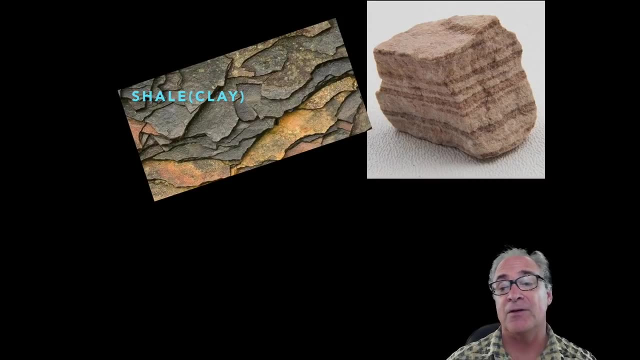 those for alluvial types of soil, especially around the rivers and the creeks here in the central valley. on this one, this one says that basically parent materials will dictate what kind of soil this is going to produce. like shale? uh, shale is basically precursor to clay materials, and then, of course, sandstone- well, sand, and then we have a basalt. 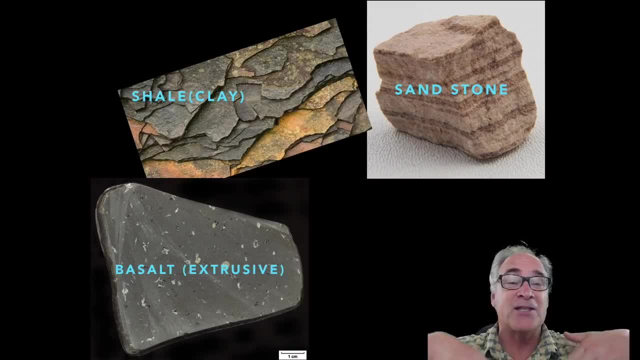 and basalt tends to, because it's extruded, air pockets get added to it as it comes out of the volcano or out of the the lava, and when it does that, those little bitty holes create avenues for water to flow, so it's a little easier to to weather, whereas granite, on the other hand,